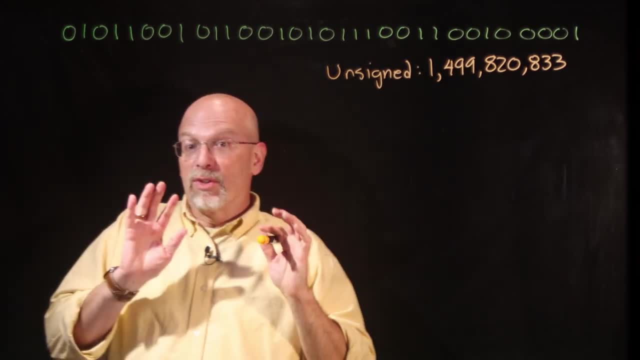 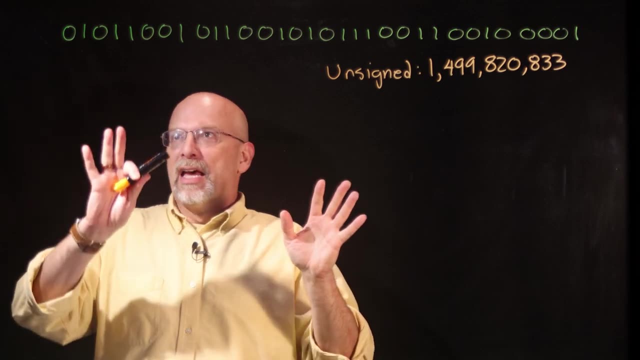 Okay, now it could be signed. Now, if it was signed, what that means? two's complement. We'll just talk about two's complement. If it was two's complement, then this could be a positive or negative number. This most significant bit would identify it as a. 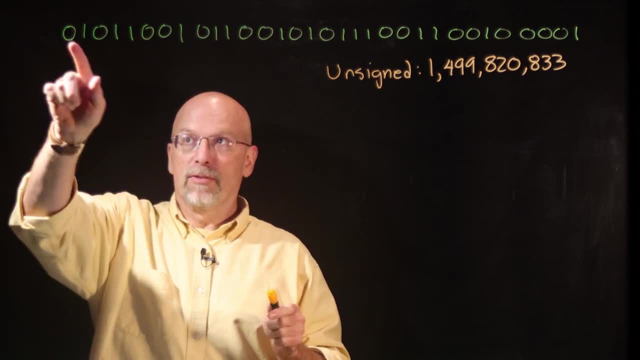 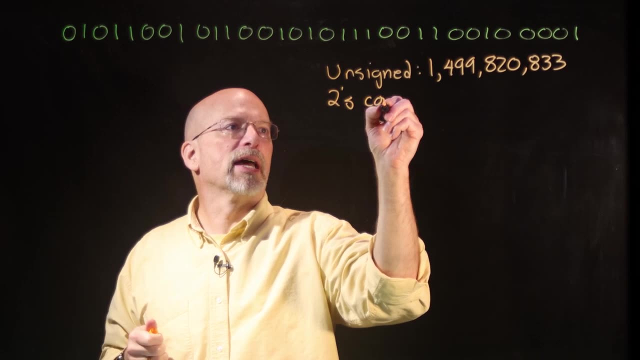 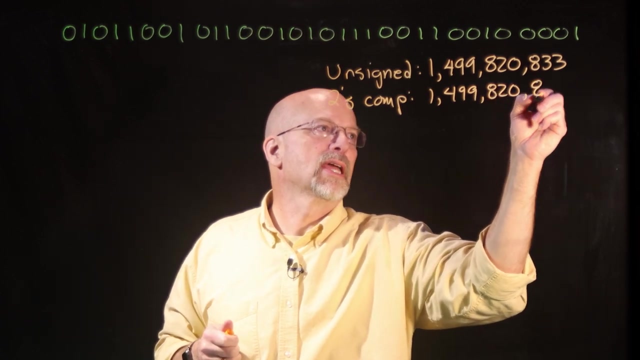 positive number if it starts with a zero, a negative number if it starts with a one. Fortunately it starts with a zero, So actually two's complement is the same as unsigned. So the two's complement will also be 1,499,820,833.. Okay, What if it is biased? 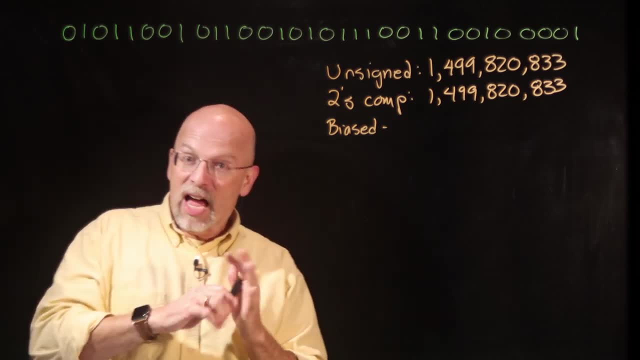 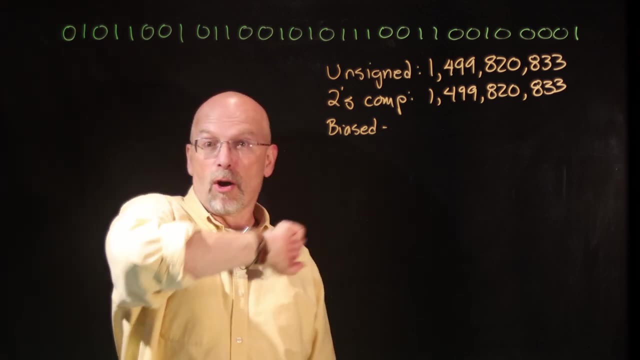 or offset. Now, if it was biased a lot of the time. what we do with bias? if we have a certain number of bits, we take the power of two of this bit and make that our bias or our offset. So this is the. 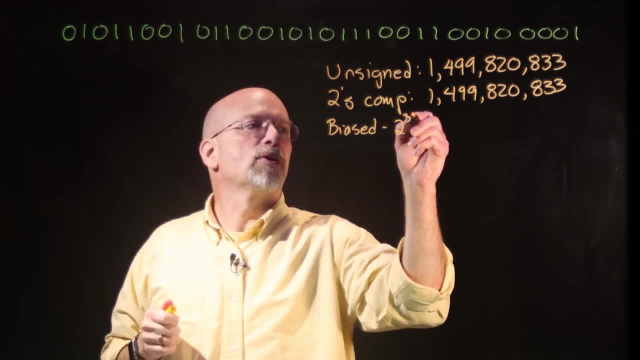 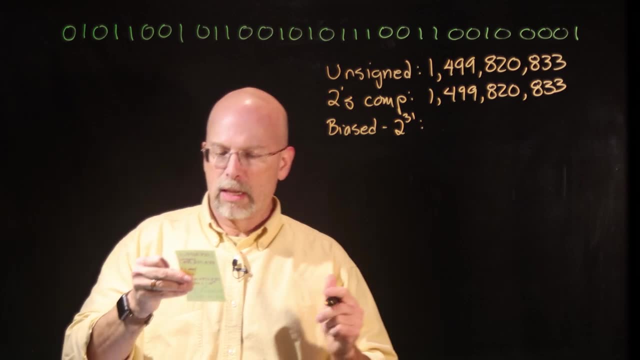 2 to the 31 position. So bias 2 to the 31.. Wow, That'll give us a negative number. Let's see That negative number would be- oh, let's see, We figured this out- Negative 647,. 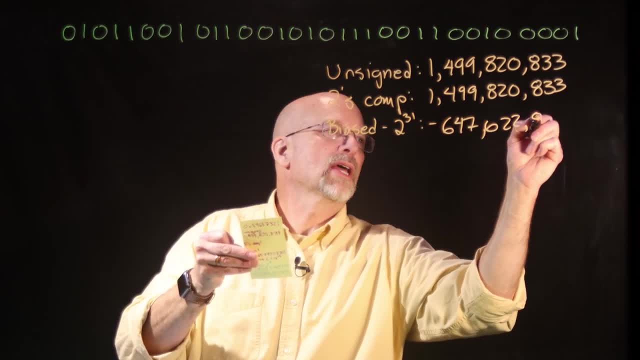 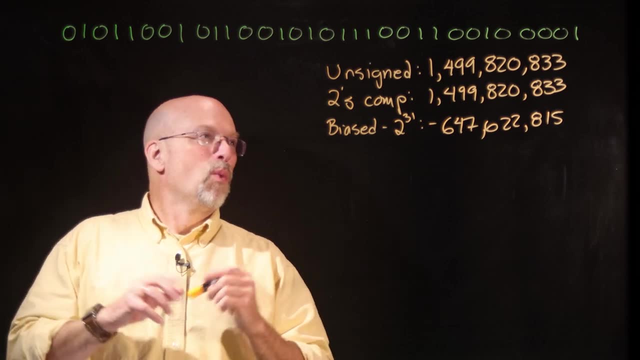 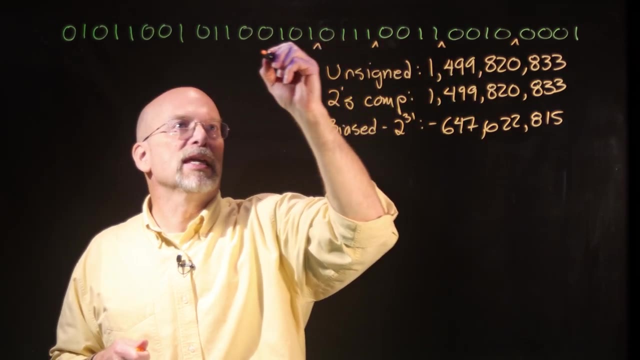 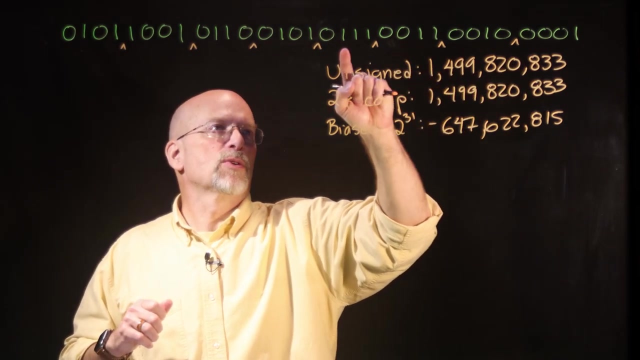 622,815.. So still a pretty big value. What if this was BCD? In BCD, remember, we divide this number into nibbles and each nibble identifies a different decimal digit. So this would be the ones place, the tens place, hundreds thousands, ten thousands. 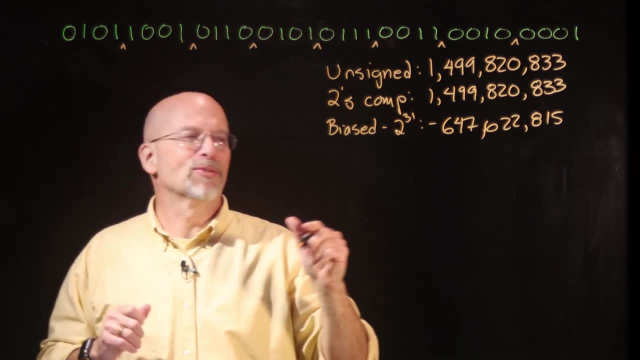 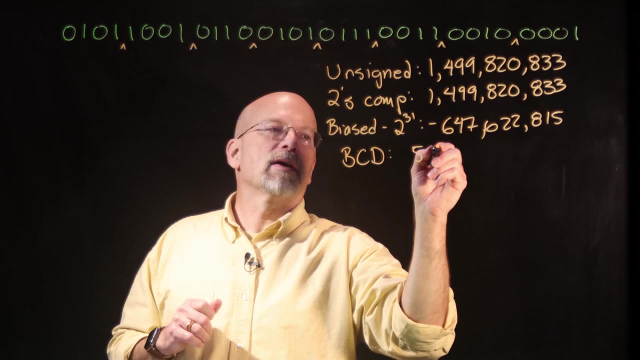 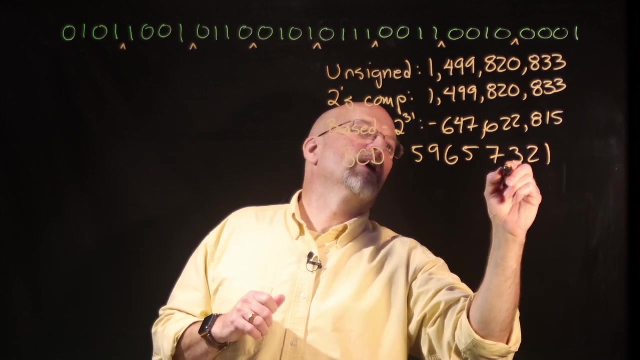 hundred thousands, millions, billions, ten millions, right. So in packed BCD this would be 5, 9, 6, 5, 7,, 3, 2, 1.. Put our commas in the right place. 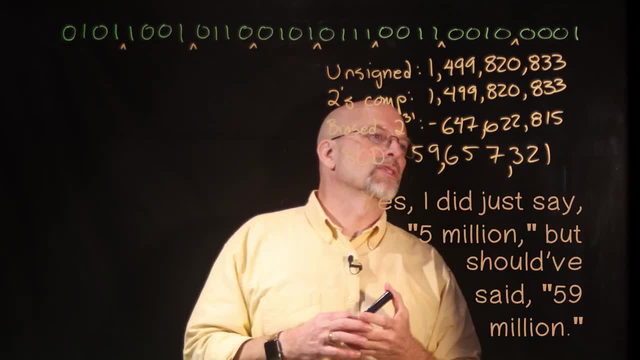 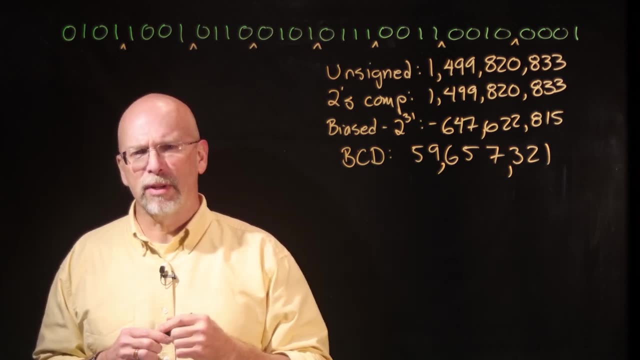 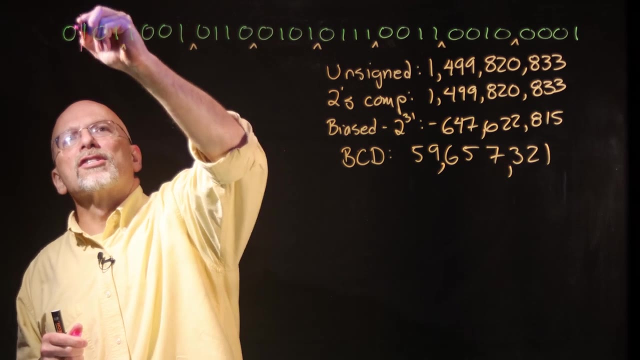 5,657,321.. What else could this be? Turns out could be IEEE 754 floating point notation, And if that's the case, well, remember, this is our sign bit S. the next 8 bits 1,, 2,. 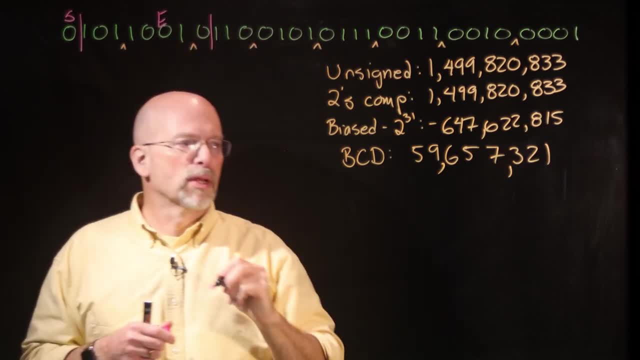 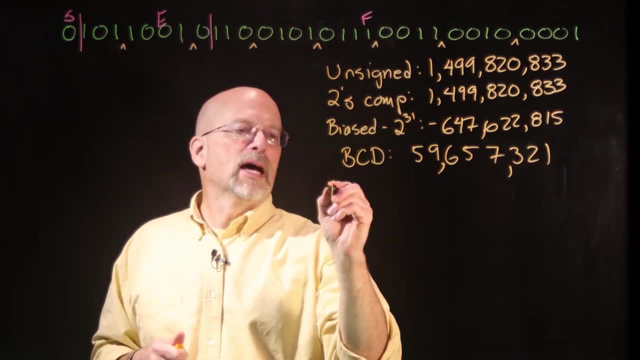 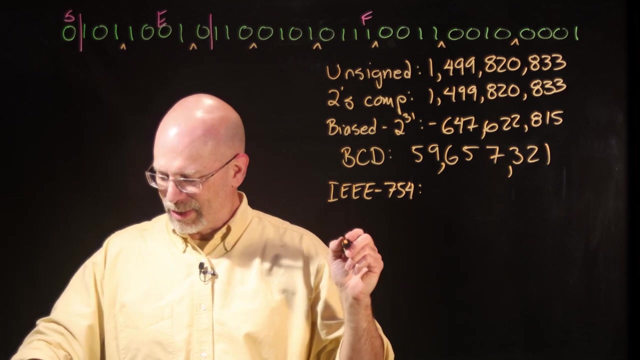 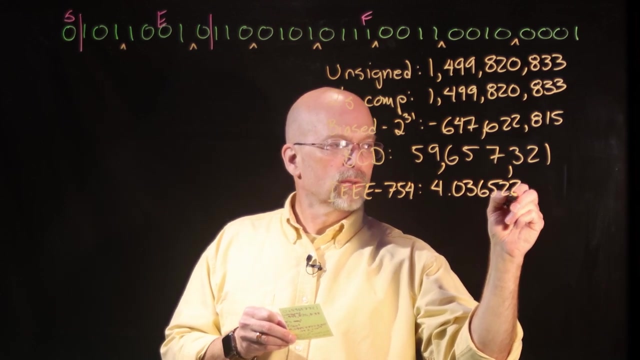 3,, 4,, 5,, 6,, 7, 8.. This is our exponent right And then the rest of it. this is our fraction. So in IEEE 754, this guy could be- I also did this calculation- for us would be 4.0365222,. 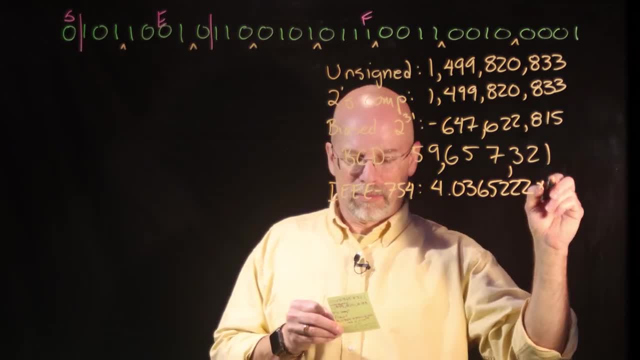 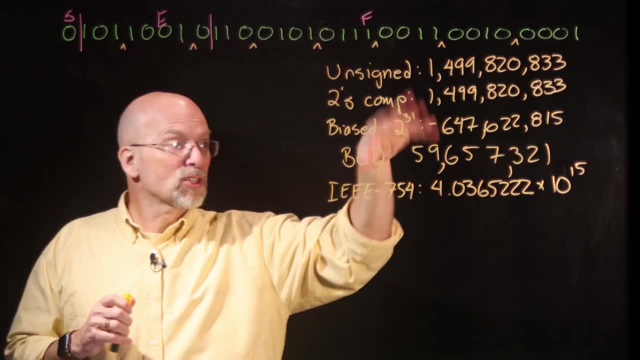 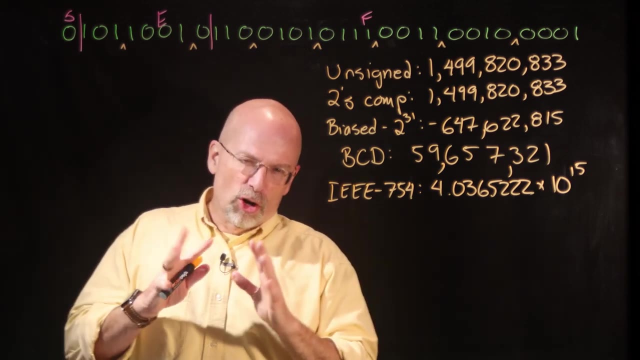 and a heck of a lot more digits, times 10 to the 15.. So there are a number of ways that this could be represented, But you notice, all of those are numbers, right? We haven't even talked about letters yet. Now, in the 1960s, early 1960s, a group of people got 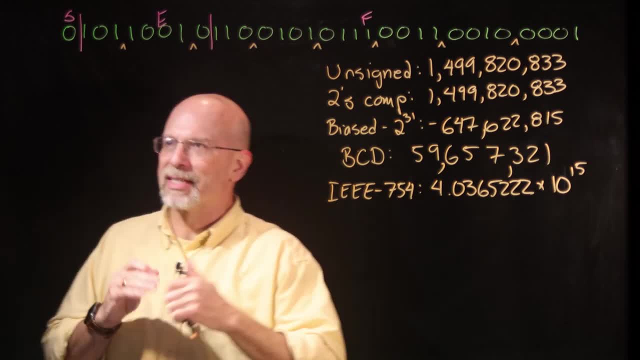 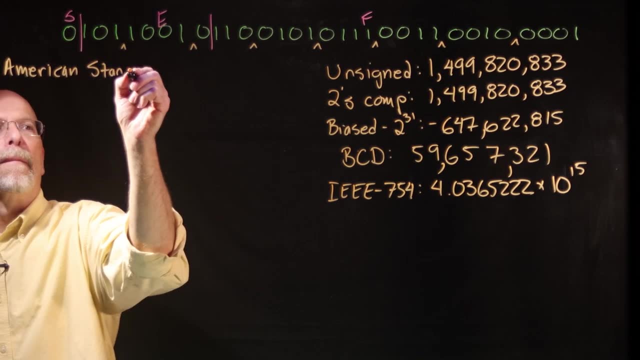 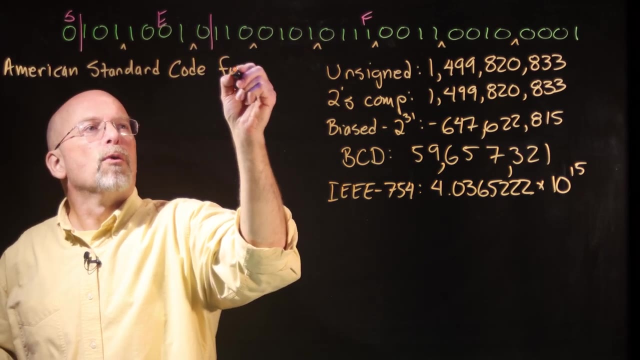 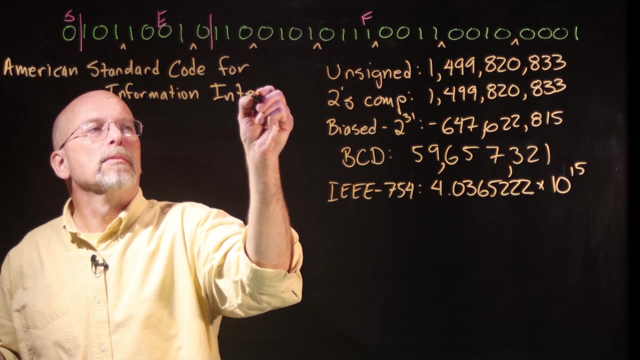 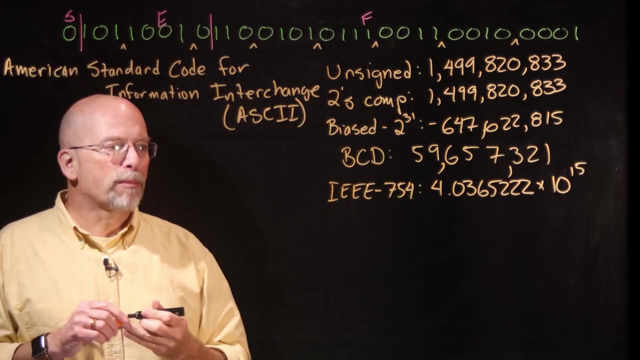 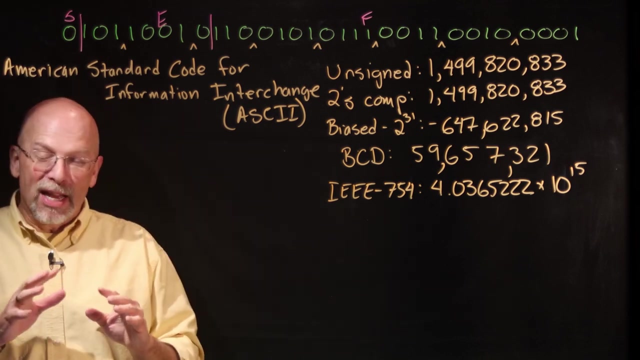 together and came up with something, and we'll go ahead and write this down. This would be the American Standard, and it's a code for information change, Otherwise known as ASCII. Now, there's an important thing to understand about ASCII, and it's this first word: American. It doesn't mean that nobody else could use it, It's just that. 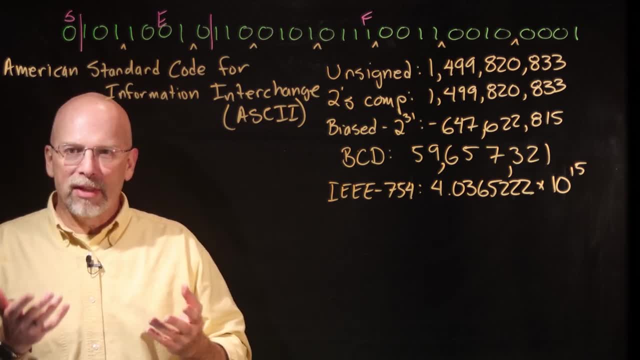 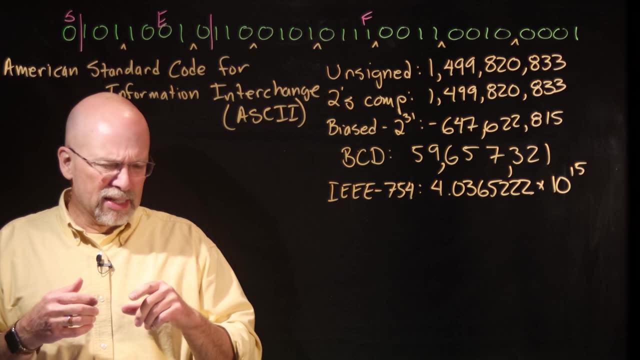 well, Americans only have 26 letters in the alphabet and it's that ABCs. And in other languages like Spanish has Enya and German has the SA And there's all sorts of other characters. but this didn't account for that, because 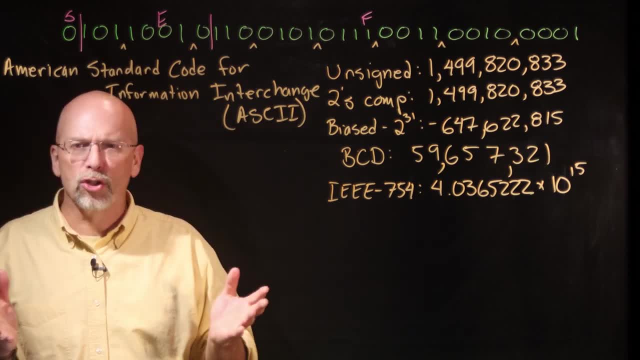 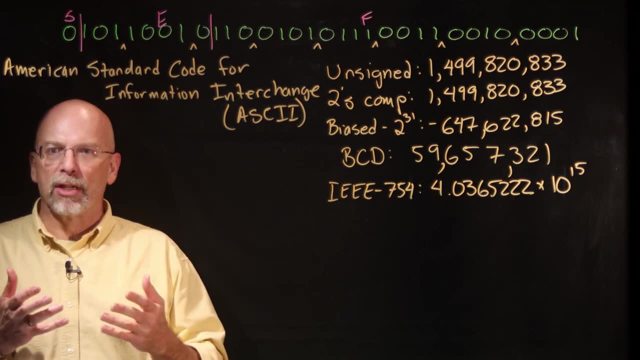 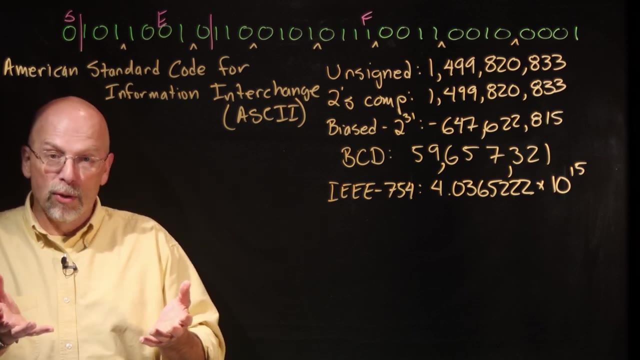 and please understand, this was not meant to be exclusive. It was just meant that back in those days it was never dreamed that we would interchange information. There were no cell phones, There was no internet. There was basically if you had a program running on. 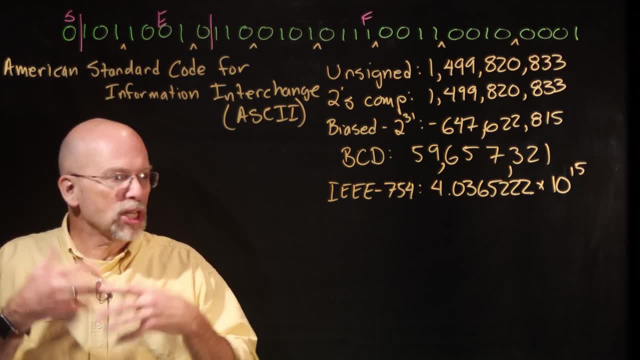 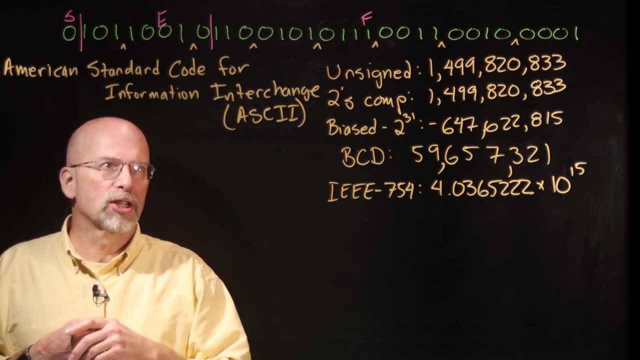 your computer. it was running on just that machine. There was no interchange with other devices. So American Standard Code for Information Interchange. And what they did was they said what we're going to do is we're going to take these patterns of ones and zeros, and we are. 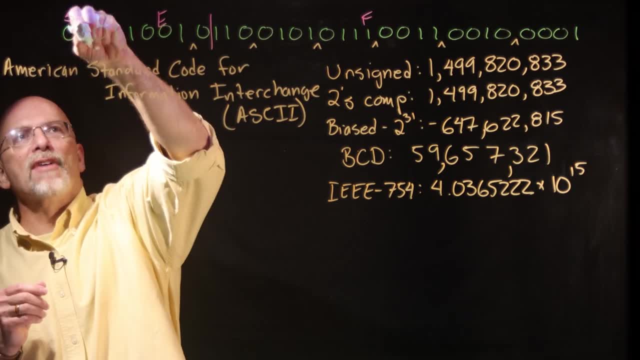 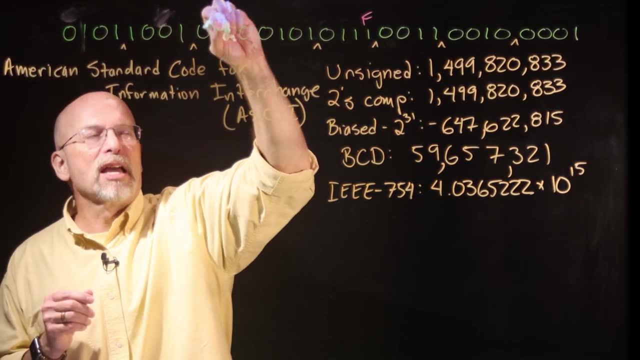 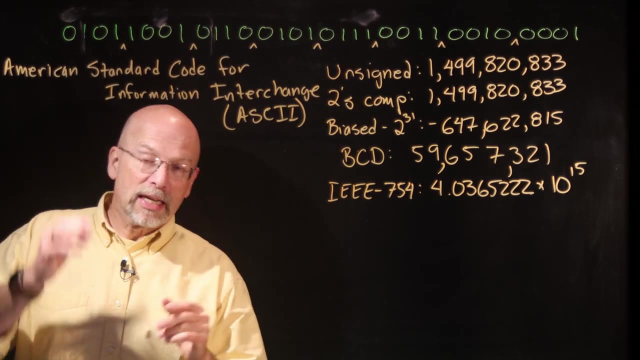 going to have them represent characters And in fact, what's interesting about this is that they figured out that if, after they kind of put together all of the characters that they thought they would need to represent, they really only needed to have seven bits to represent a character. 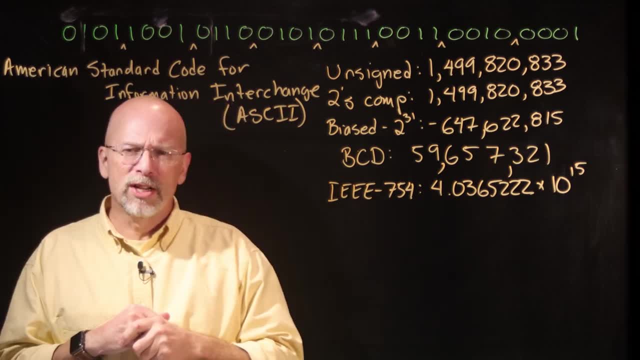 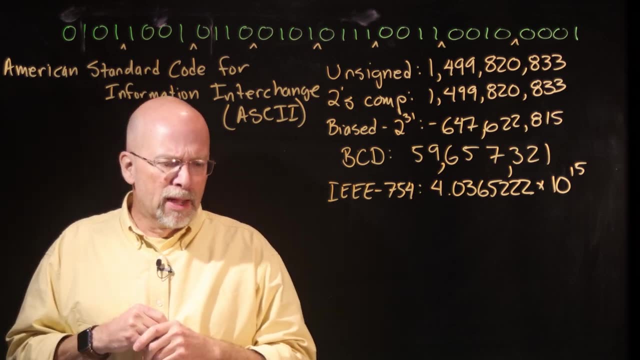 Think about this. There were like 25 punctuation marks and mathematical symbols and space and carriage, return and line fade, things like that that they would use. There were 26 uppercase letters and in fact the original standard only used uppercase letters. They didn't even worry. 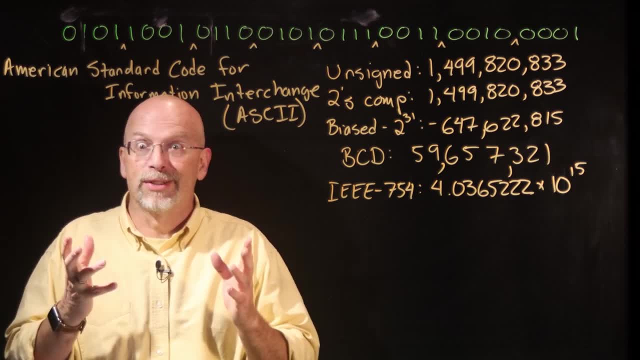 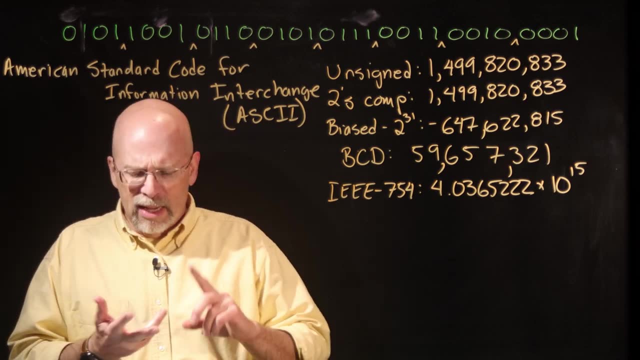 about lowercase letters. Everything was just going to be capitalized, shouting all the time. right Then there's 26 lowercase letters. So right now we're up to what? 77? Something like that. They had some control characters. 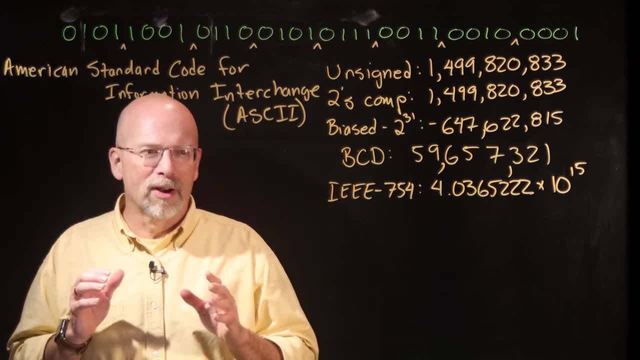 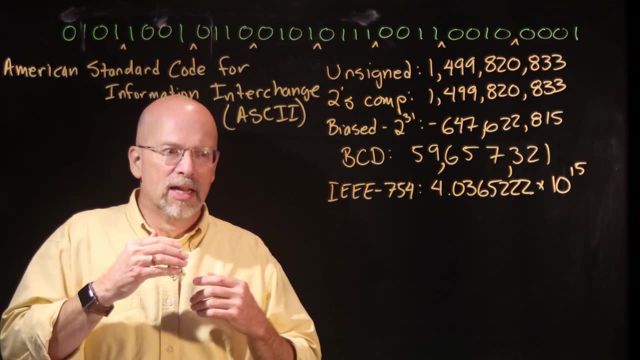 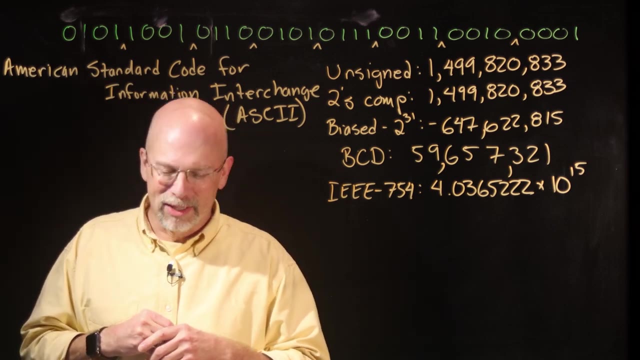 Some unprintable control characters, Everything from a null, and something that indicated that we had an end of a message, something that was indicated that there was, in fact, there was a bell. There was an audible bell to make it so that there was a ding as part of the message. 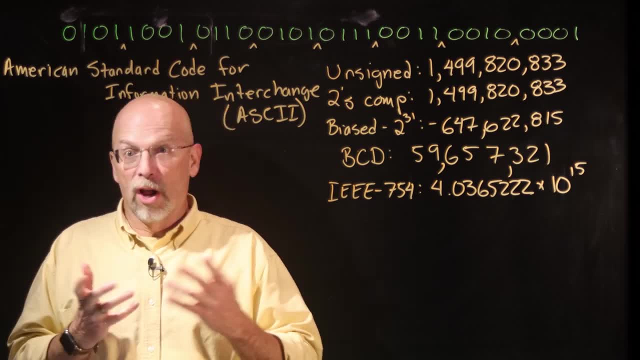 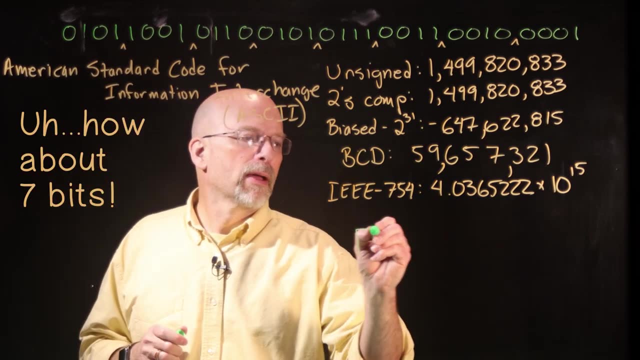 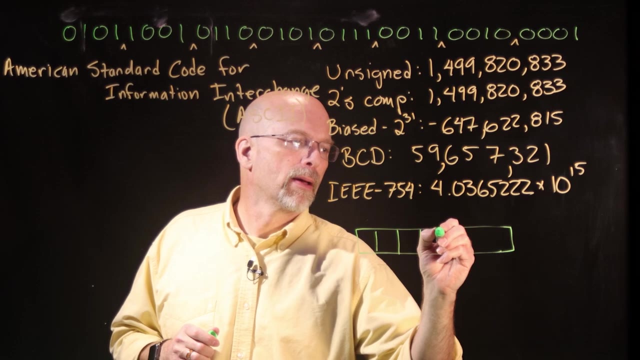 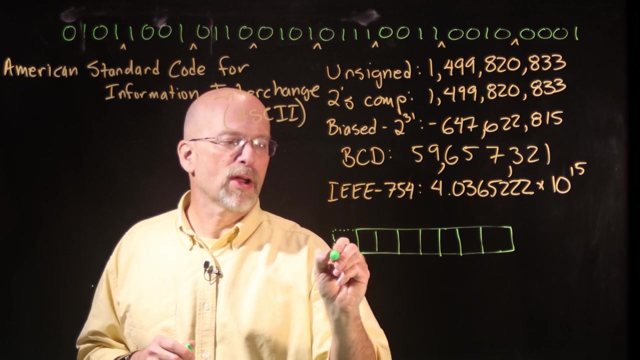 Well, that was less than 127 or 128, which was all the patterns of ones and zeros we needed for eight bits. Now, if you look, got my squeaky pen again and we divide this up into seven bits. So we have seven bits and what happens is, if we are storing or sending eight bits, 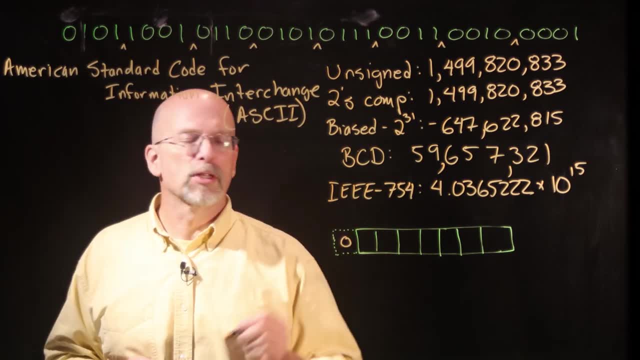 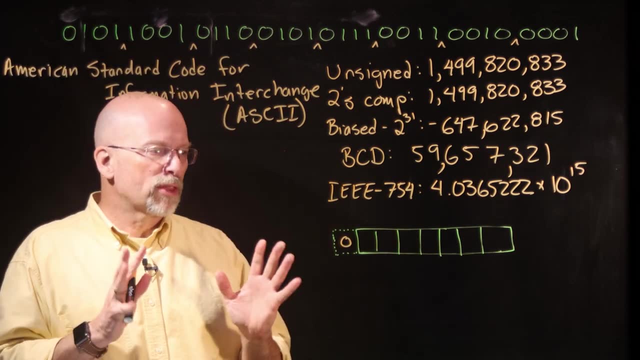 anyway, what we're going to do is we're just going to automatically assume this most significant bit is a zero all the time. all right, It is possible to communicate back and forth between machines with just seven bits, but in this case we're looking at an eight-bit, you know. 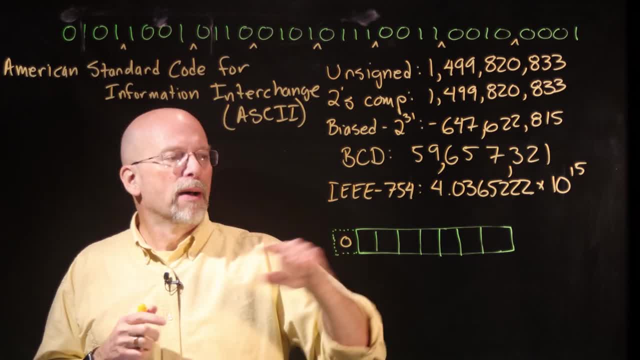 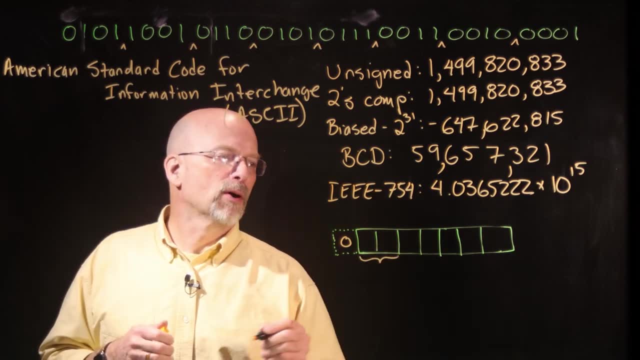 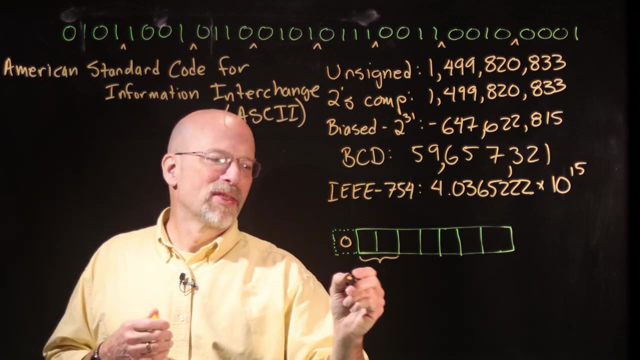 we've talked about this before. We like to do things in eight bits. This most significant bit is always going to be a zero. Now, these most significant two bits. they or, excuse me, yeah, the most significant two bits. they tended to categorize the type of character that we were. 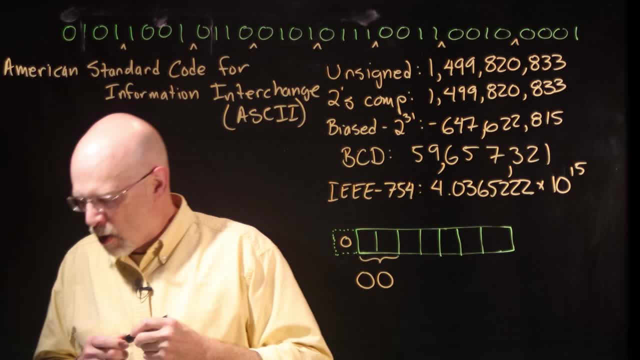 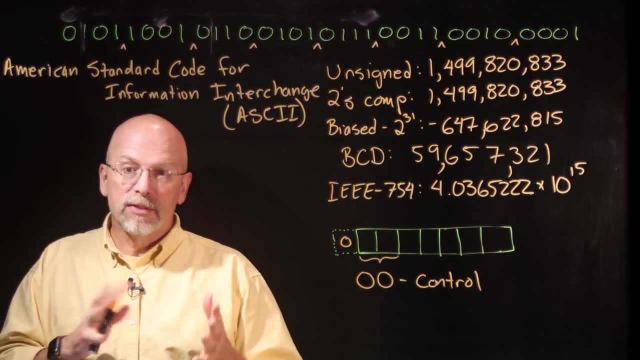 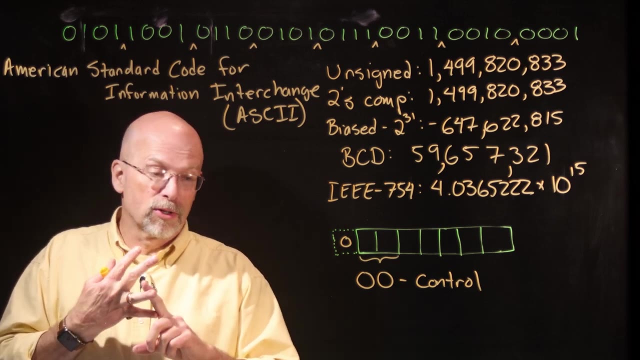 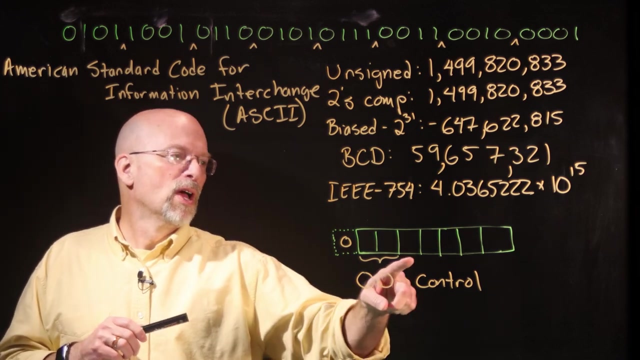 showing. So if it started with a zero zero, what you were looking at was mostly control. So this thing, like I said, is a zero zero. So if it started with a zero zero, we had. well, how many bits do we have left? One, two, three, four, five, two to the fifth. 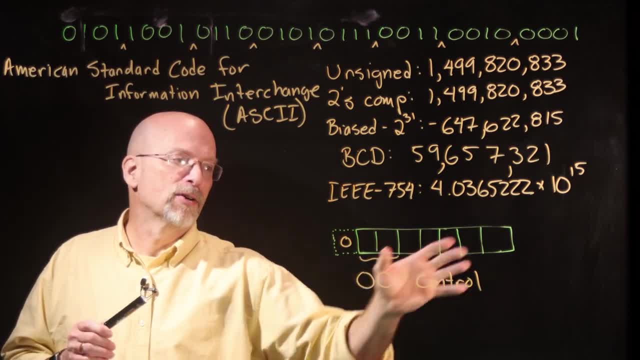 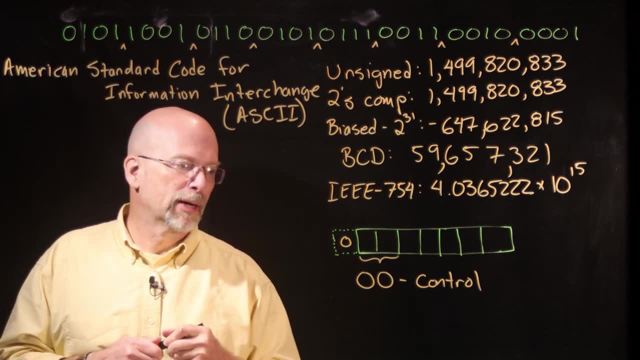 that's 32 patterns. So there were 32 patterns that would be part of those that we could use with those. all right, So if it started with a zero, zero we had. well, how many bits do we have? 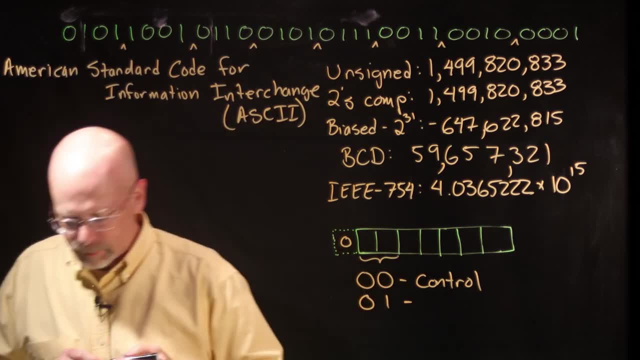 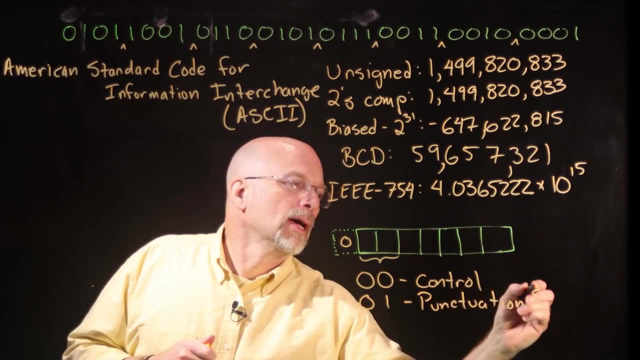 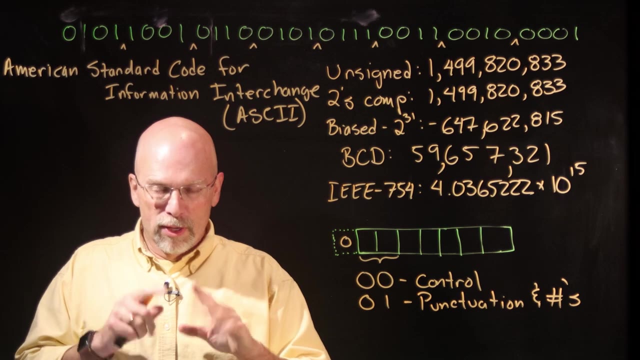 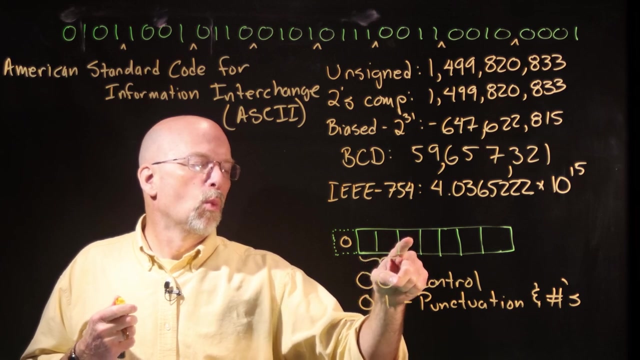 left. Now if it started with a zero one, this zero one tended to be punctuation and numbers, all right. Now the interesting thing was that numbers all the numbers, so starting with zero, all the way up to nine. So zero one and then one zero, zero, zero. 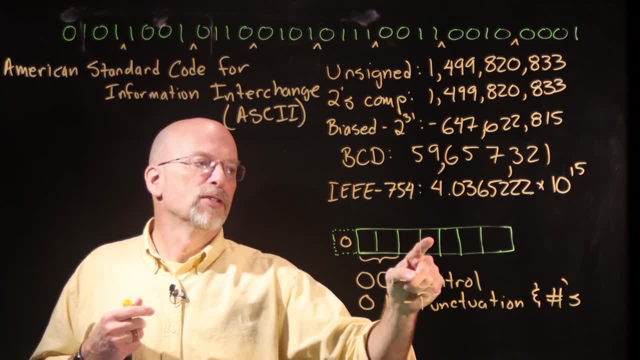 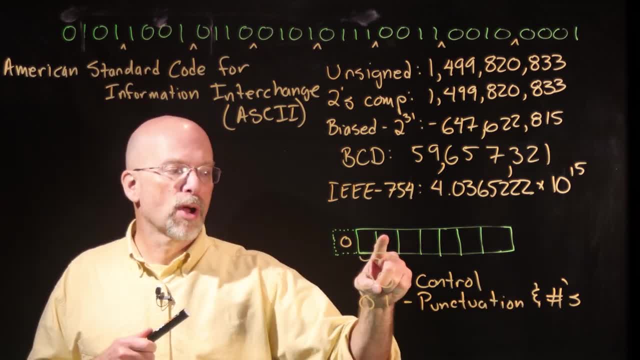 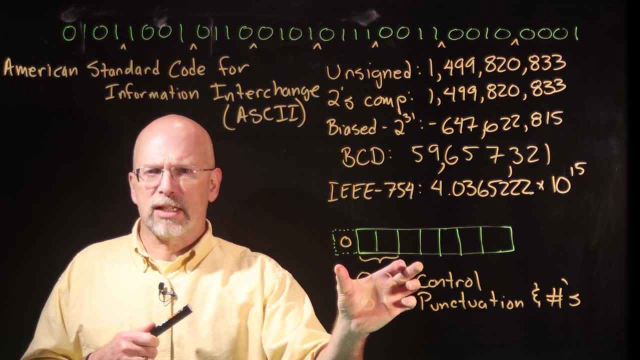 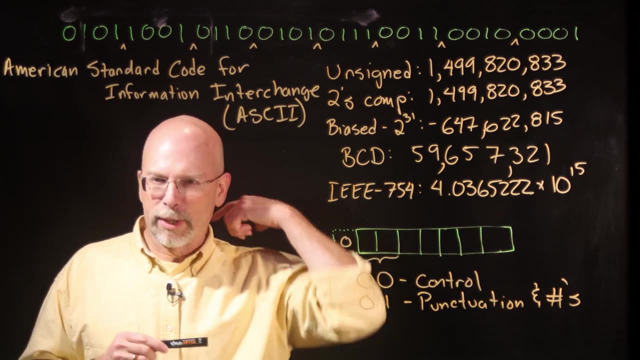 at was the numbers themselves always started with zero one, one which meant that all you had to do you notice this nibble right here was a hexadecimal three and this nibble right here was whatever the decimal digit was. So you got real used to in your programming. 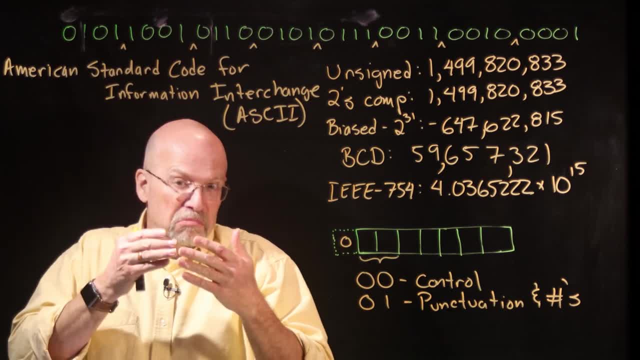 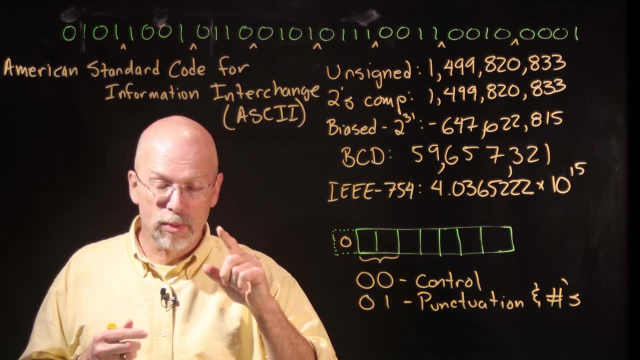 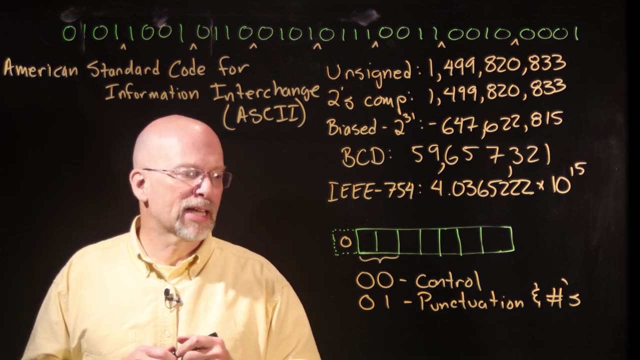 language. if you wanted to convert an actual nibble zero through nine to this ASCII, you would, All you had to do was just add a zero- excuse me, a three zero, hex to it. it would automatically create the ASCII version of that number If it started with one zero in addition to 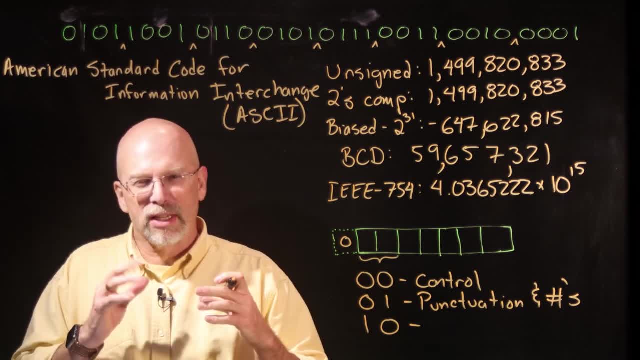 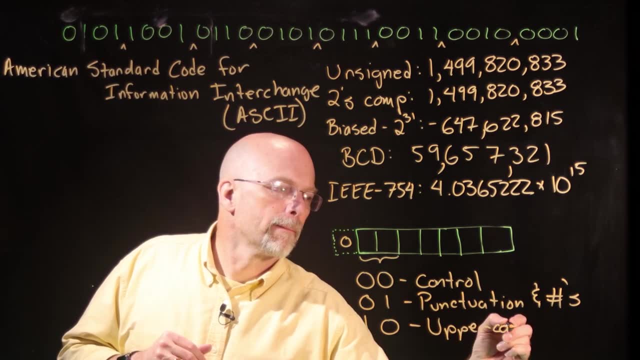 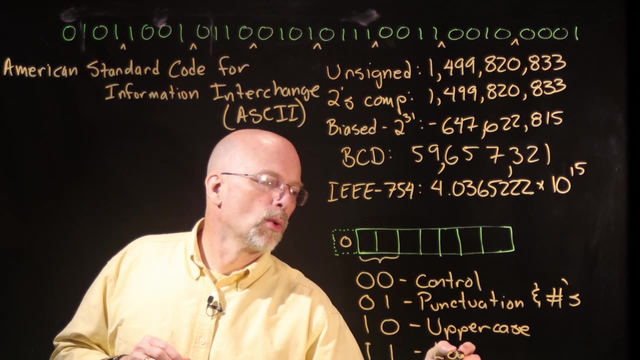 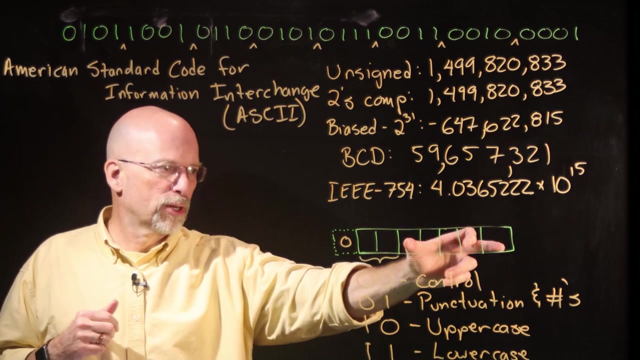 some punctuation like parentheses and so forth. this was, for the most part, uppercase letters, all right, And if it started with, If it started with one one, it was lowercase letters, all right, And some additional punctuation because, like I said, there are 32 patterns of ones and zeros there. so what we've got. 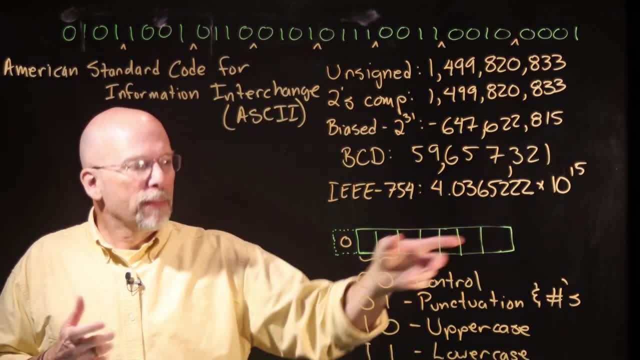 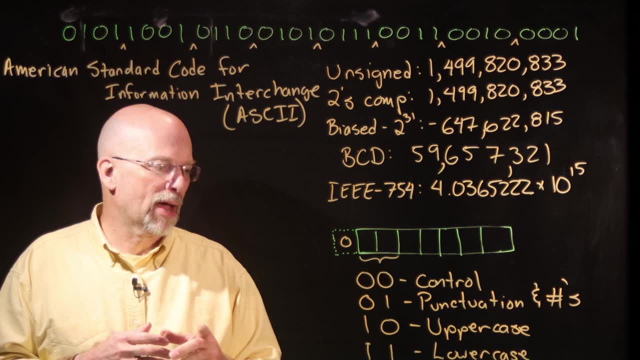 is the 26 letters A through Z, plus, you know, 10 different characters or, excuse me, six different characters. Now, something that was interesting about these things: if you wanted to change something between uppercase and lowercase letters, you would have to do this. If you wanted to change. 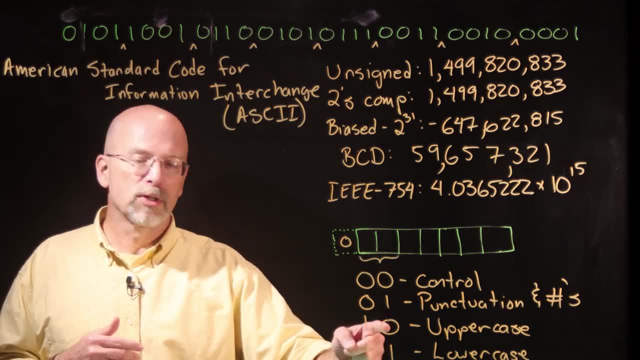 something between uppercase and lowercase letters. you would have to change something between uppercase and lowercase letters. you would have to go from uppercase to lowercase, And if it's only inflation, you're probably going to change something. All you had to do is either turn this guy a bit to a zero or turn that bit to a one, Just flipping back. 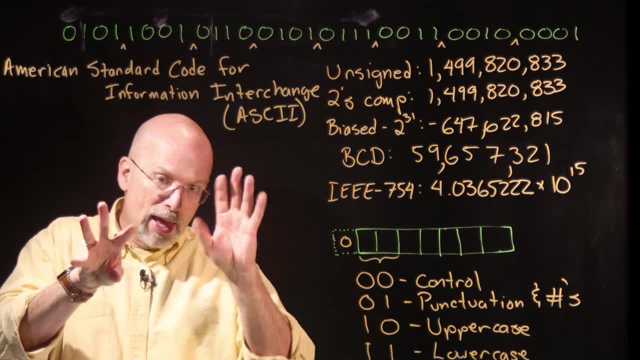 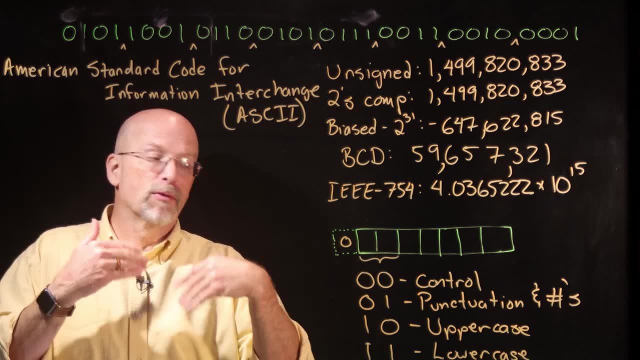 and forth between zero and one, the letters, the capital A and the lowercase, a lined up with those bits. just fine, All you had to do was just clear or set that bit in order to go from uppercase to lowercase, And so it should not get complicated. 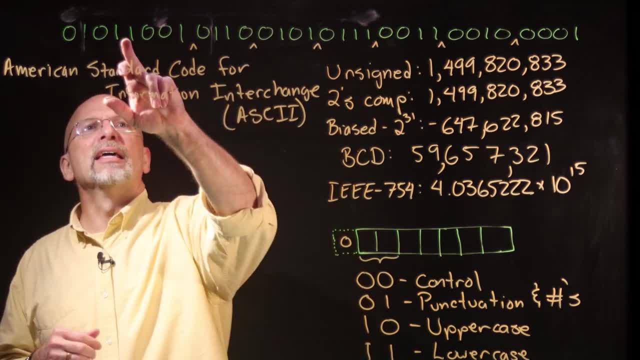 Alright. So let's take a look at this number again, And I realize things have gotten a little messy from whenever I first put this up on the board. So what can we do about that? Here's three number lines, four important and five important pieces. You have four. 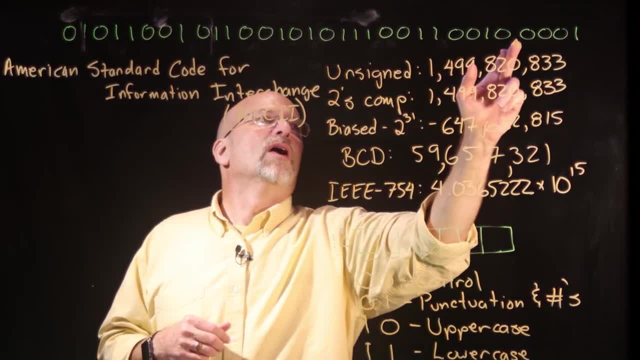 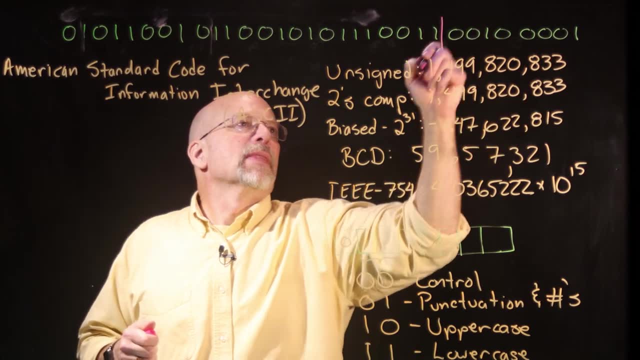 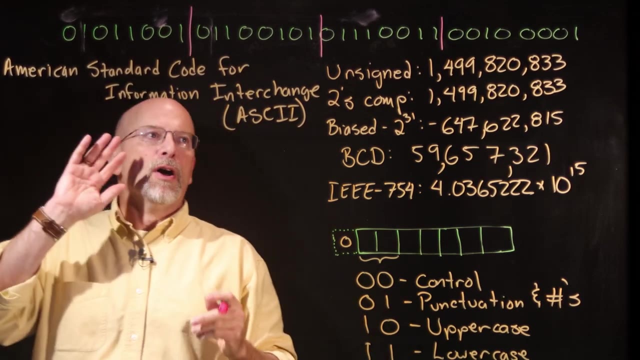 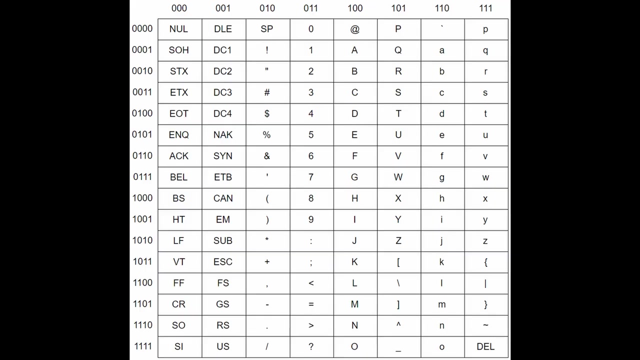 but let's see what we can do with it Now. let's assume that now what we've actually got is eight bits, eight bits, eight bits and then eight bits. All right, now what you can see, and in fact, let's take a look at an ASCII table. This ASCII table that we're looking at right now. it shows: 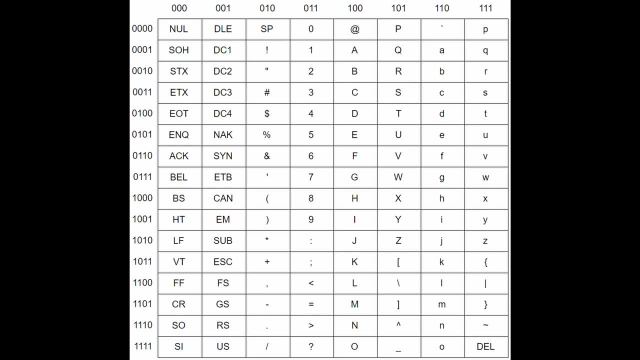 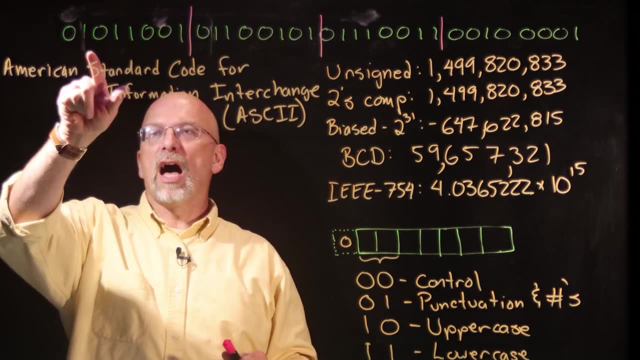 you in the columns the most significant three bits of the ASCII value and the rows are identified with the least significant four bits of the ASCII value. so you've got the seven bits total. So if we look at this first value and we go over to column or- excuse me, we'll take a look at the. 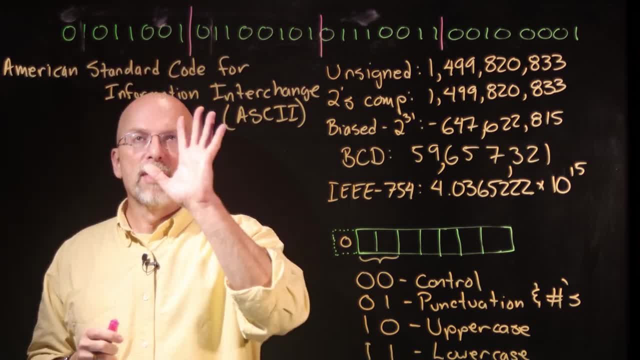 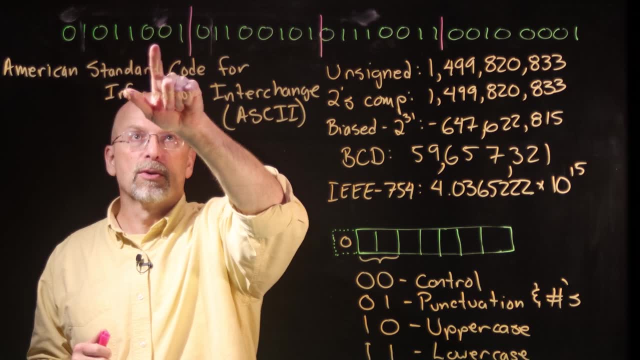 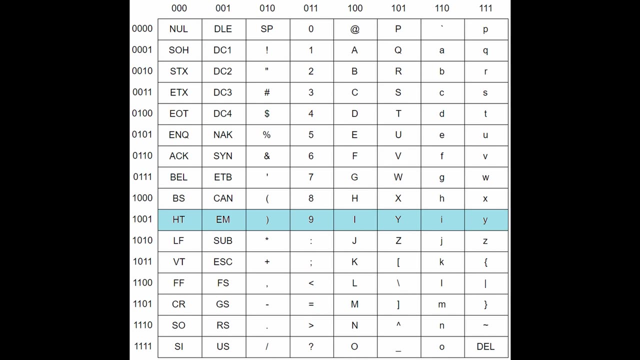 the rows. first we look at the least significant four bits of that first byte. that first byte is one zero, zero one. those last four bits of that first byte: One zero, zero one. we go down to the ninth row, or the one zero, zero, one row. Okay, that row. we then 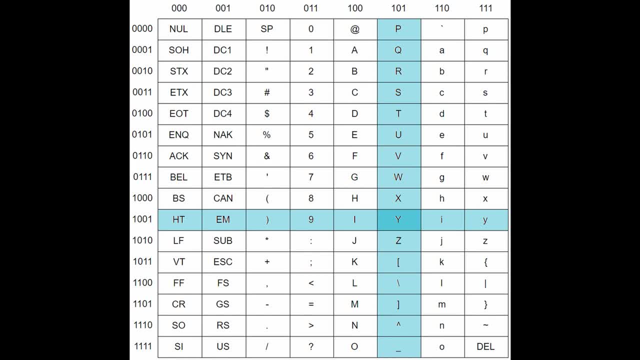 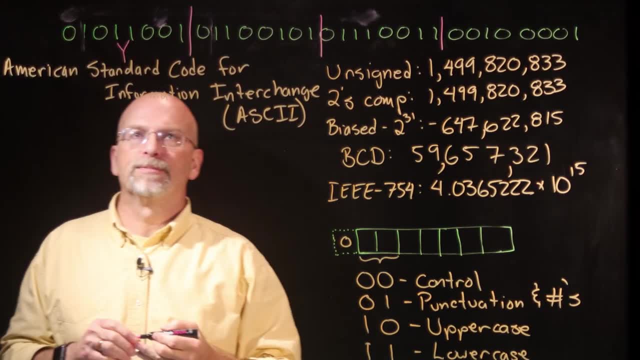 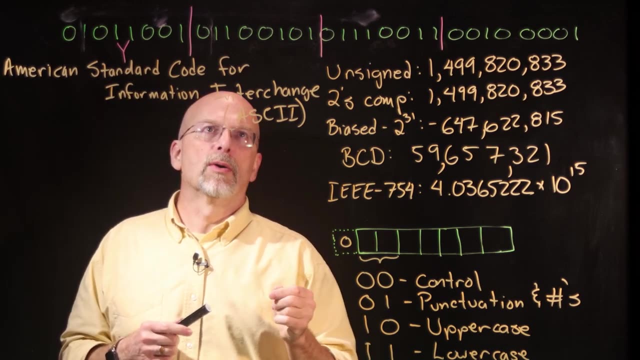 follow across to the column one zero one and then one zero one, where those two intersect. we see that this is a capital Y. All right, capital letter Y. Let's look at the next byte. The next byte is zero one. one zero, zero one zero one. All right, let's once again. 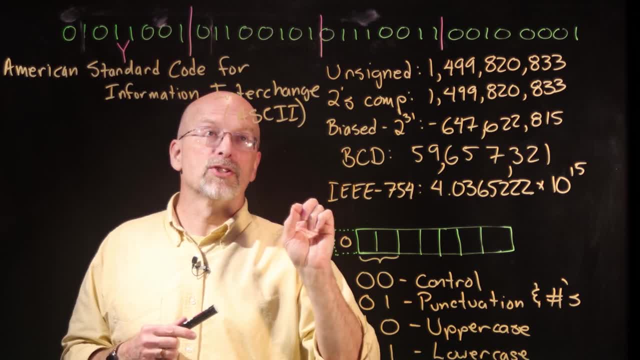 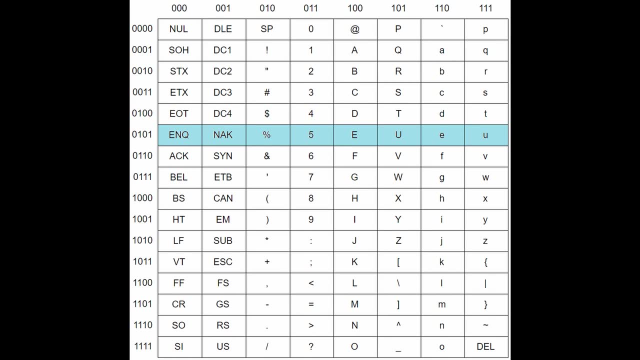 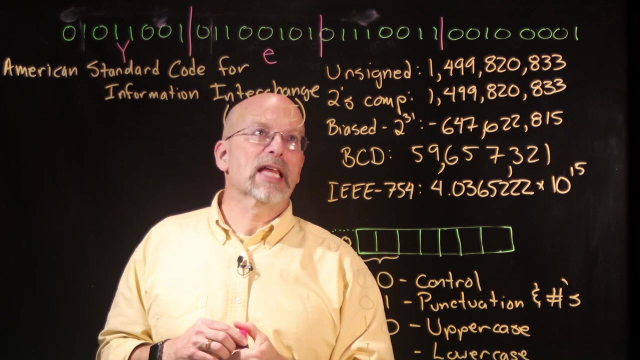 Start with the least significant four bits: the zero one, zero one. We go down the rows until we find the row identified by zero one, zero one, and go across until we get to the column identified by one one, zero. That gives us the lowercase e. The next, the next eight bits, the next byte. 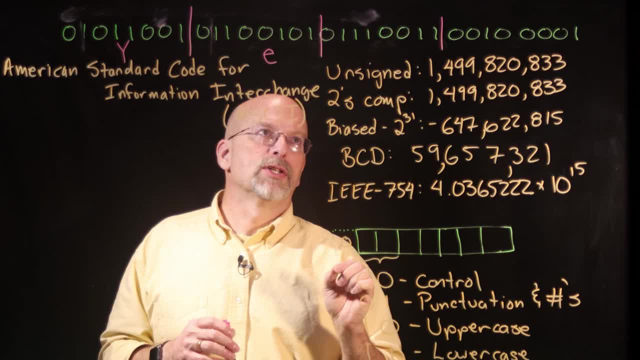 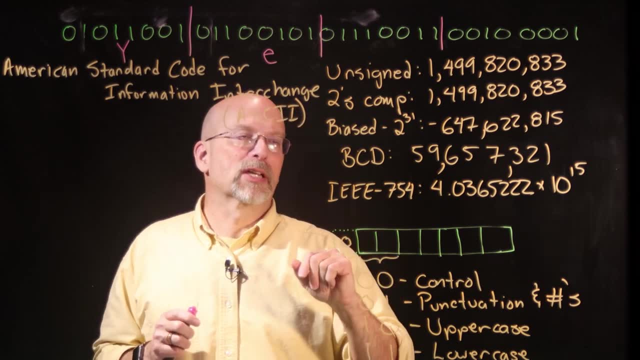 the next byte is zero one one one, zero one, zero one, zero one, One, zero, zero, one one. And in fact we can go back and talk about you know what I'd with those most significant two bits. The most significant two bits of those seven bits are one one. So we know. 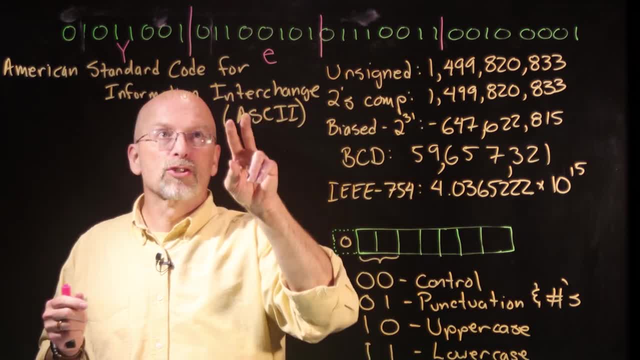 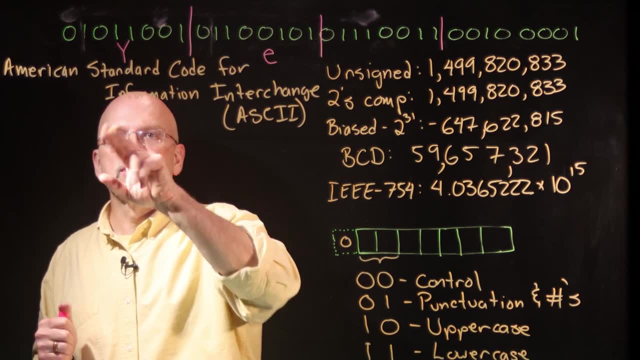 this is going to be a lowercase letter. The previous byte, the most significant two bits were one one. We knew that was going to be a lowercase letter and it turned out to be a little e. The first one. the most significant two bits of the seven bits are one zero. That gave us a capital. 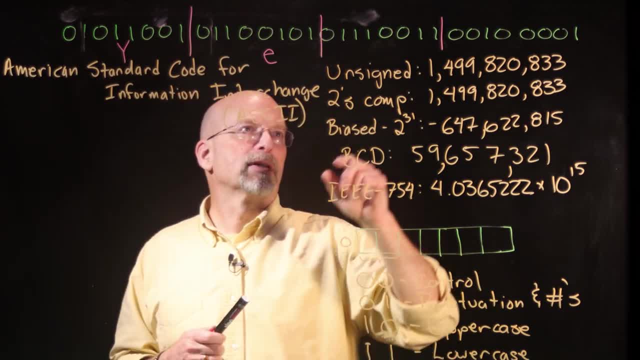 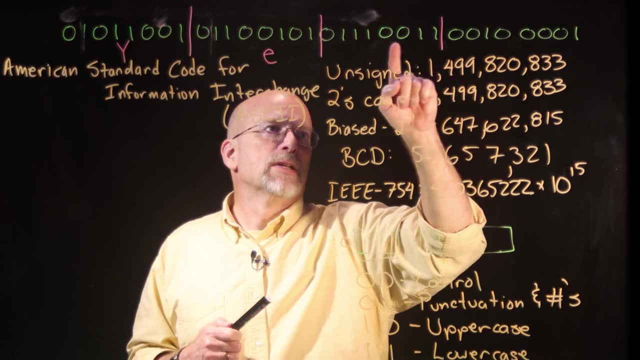 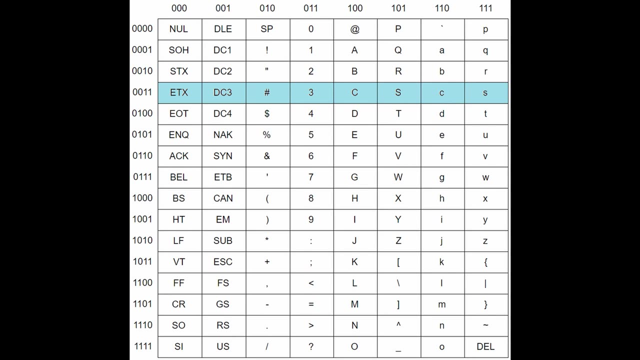 letter, a capital Y. Now getting back to this third Byte, the last four bits of the seven bits are zero, zero one one, zero, zero one one. We go down the row and then go across until we find the column identified by the most significant three bits of. 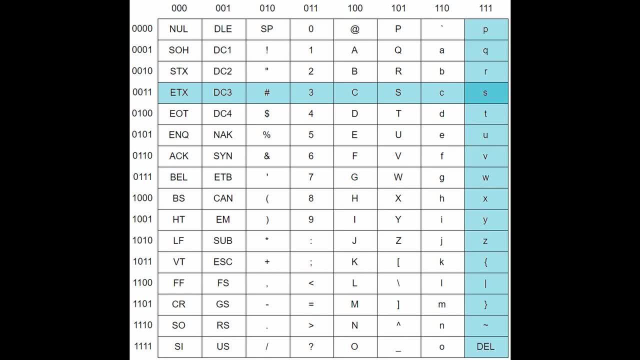 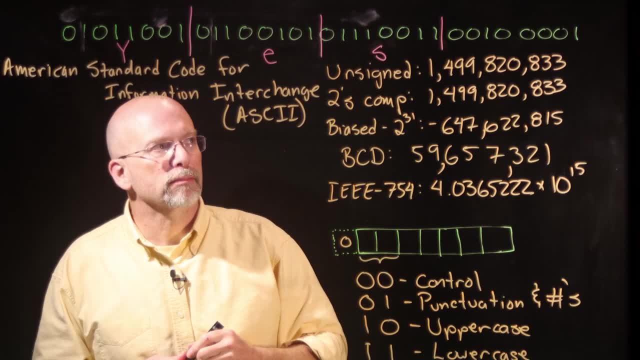 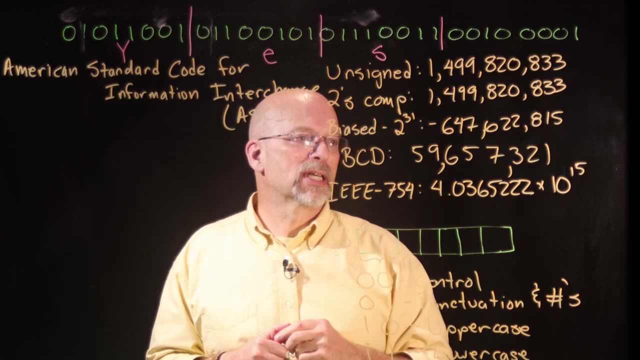 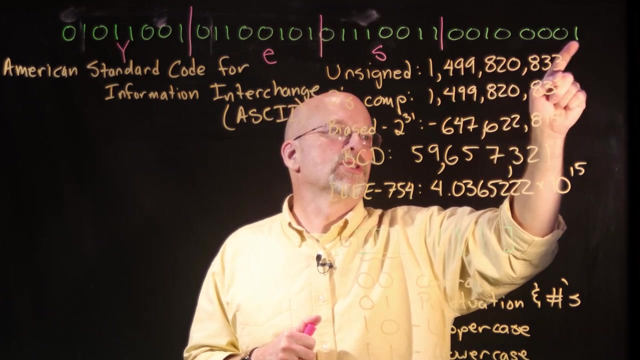 those seven bits. one, one, one, one, one one gives us the last column where we see a lowercase s. Now let's look at the last column. Now, let's look at the last column, The last byte, the last byte. take away that most significant zero, that most significant bit zero, and we've got the seven bits: zero one, zero, zero, zero, zero one. 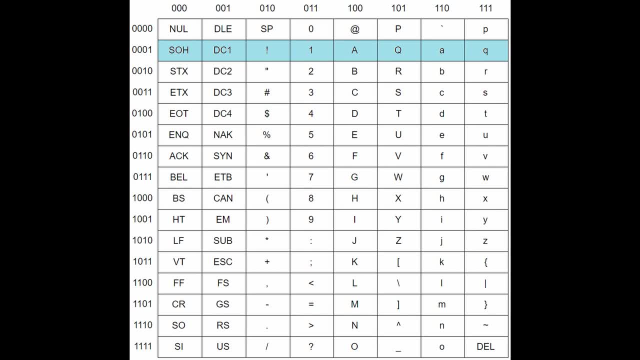 So we go down to the row zero, zero, zero one- That's the second row down- and then go across and notice the most significant two bits of those seven bits are zero one, which means it's a punctuation or a number. We go across to the column identified by the most significant three bits. 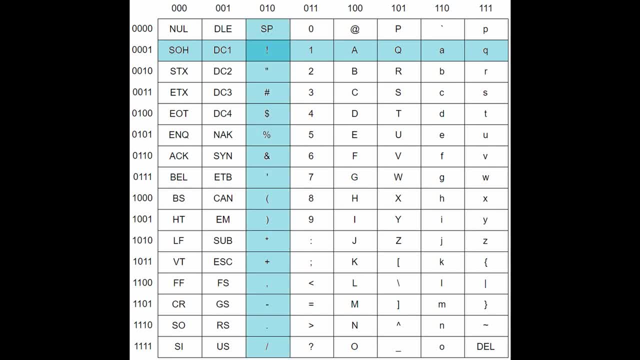 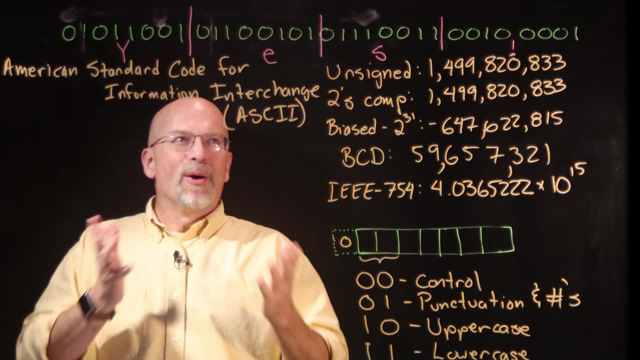 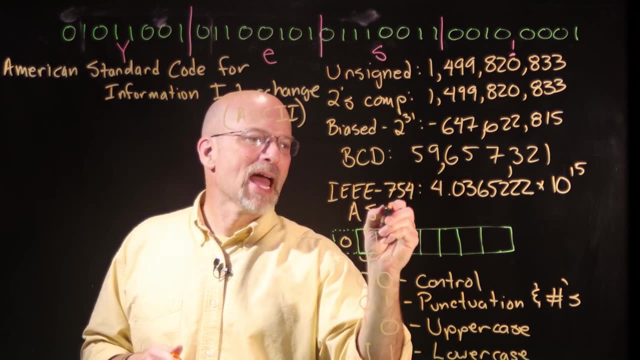 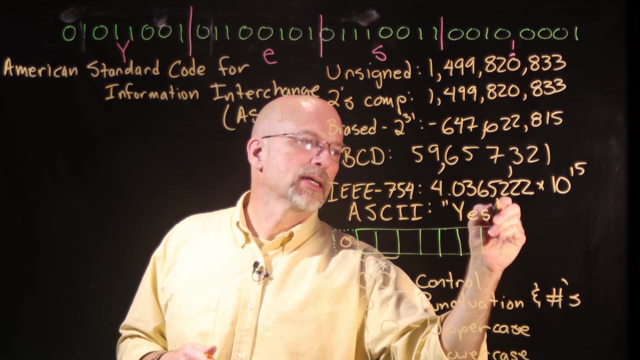 We go across to the column identified by zero, one zero, and we see an exclamation point, the punctuation that we're looking for. All right, All right. So these thirty two bits in, and let's go ahead and write this down in our last bit in ASCII, represent the text string capital: Y little e little s exclamation point. 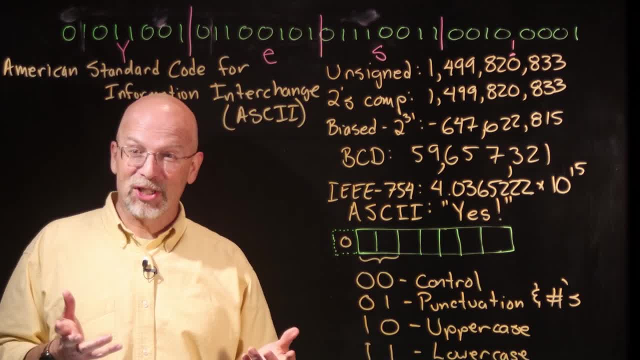 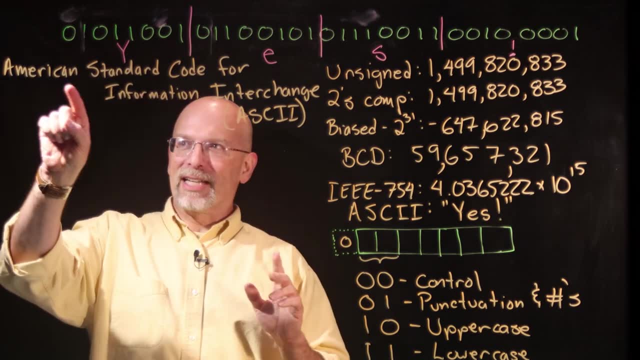 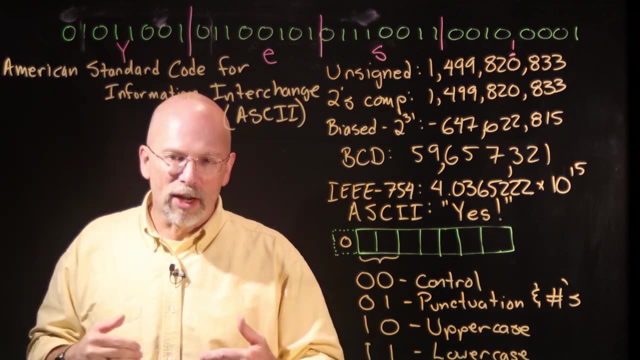 There you go Could have represented that too. Kind of looks like it did. Now, the key thing that we were talking about with this is that term American. We're going to see how the ASCII was a starting point For something we call code, points with something we call Unicode.